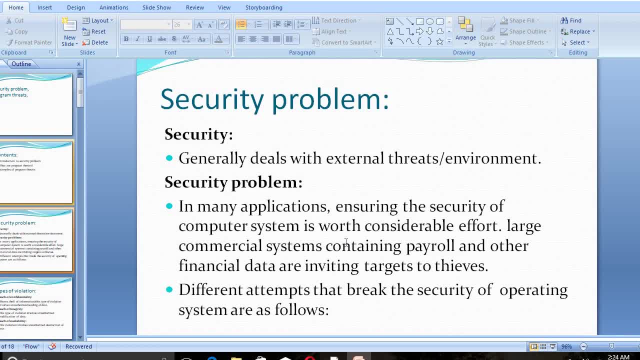 security. What is security? Security generally deals with external threats or environment. External threat means unauthorized person try to access the system. Security problem In many applications. ensuring the security of computer system is worth considerable effort. Commercial system- mostly payroll or financial data to access. 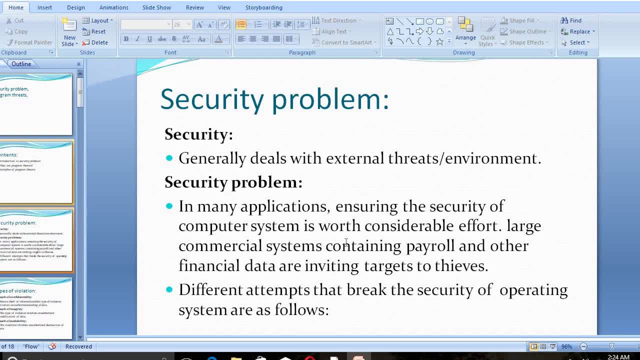 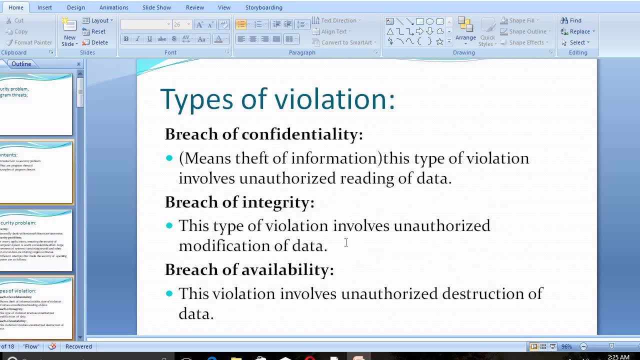 the system. In many applications, the target of malicious user is to access the system, So they make different attempts to break the security. Here are the different attempts. First, breach of confidentiality means theft of information. This type of violation involves unauthorized 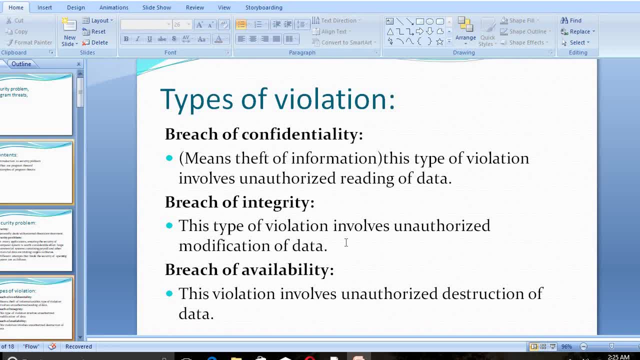 reading of data As impact will be affected by a malicious user. If a malicious user tries to access the data in a system is called breach of confidentiality. Breach of integrity means unauthorized modification of data In a Trick code file using malware. a user experience, some analytics expression: 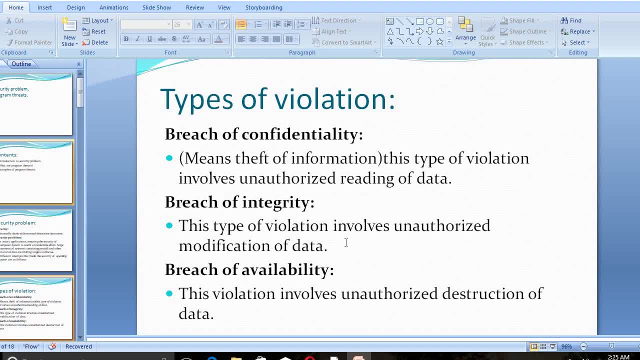 For example, if a malicious user tries to modify the data in an unauthorized way, they have to sweetness by querying the local data scarce, called breach of integrityion. For example, if the malicious user tries to modify the data in an unauthorized way, it's gear to the much more unsuitable way. 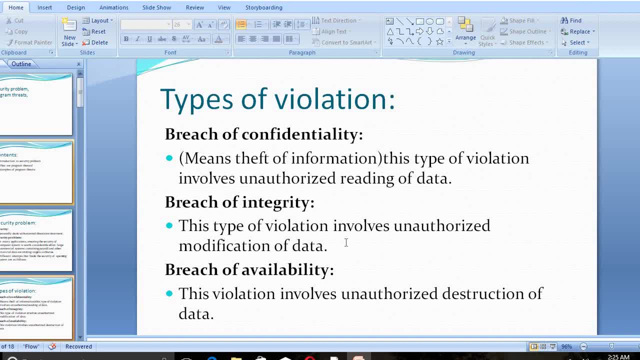 This is called breach of Integrity. Breach of Availability is. the best way to manage data release is to reduce time скratch and run out data, for example, means unauthorized destruction of data. For example, F1 and F2 are two resources of operating. 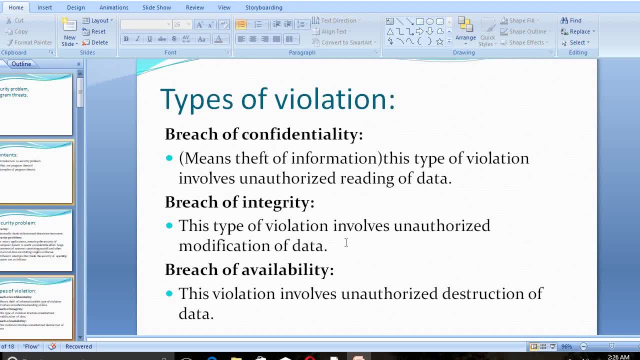 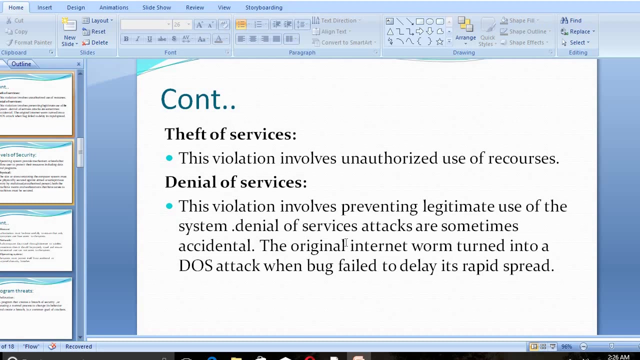 system and D1 is a process that have access to F1 and try to access to F2 and X is a malicious user that modify in F2 before accessing the D1 process, which is called breach of availability. Theft of services means unauthorized use of resources, For example, D1 is a process and 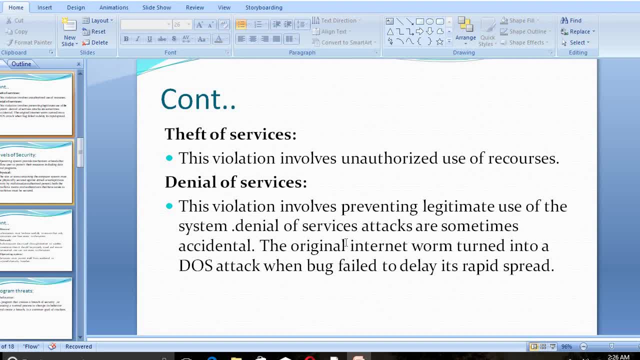 F1 and F2 are two resources of operating system. F2 are the resources and X is a malicious user which have access to F1 and F2 and consume all resources of F1 and F2 for destruction And now process. D1 cannot access these resources. 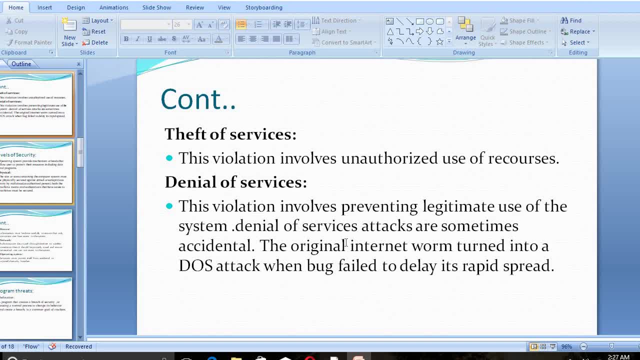 which is called theft of services. Denial of services means unauthorized use of resources. This violation involves preventing legitimate use of system. Means denial of services. attacks are sometimes accidental Means internet through worm or any type of viruses are interred in the system. 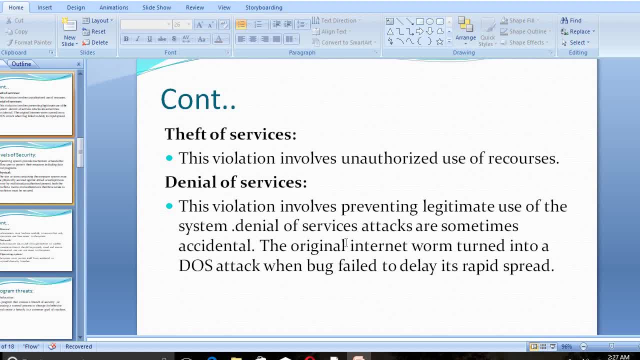 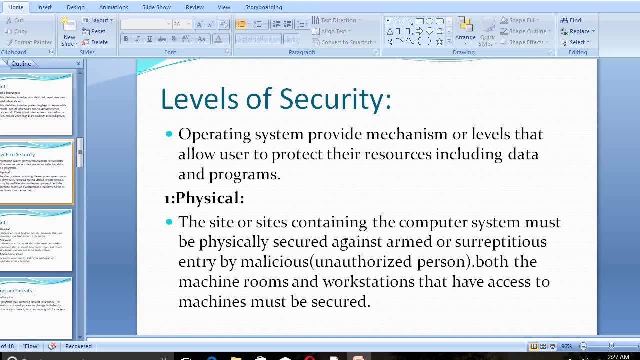 System is interred in the system. System is interred in the system. Now we have finished discussion about the safety of system and its operating systems. Let's talk about what we call denial of services. Now we have come to the level of security. 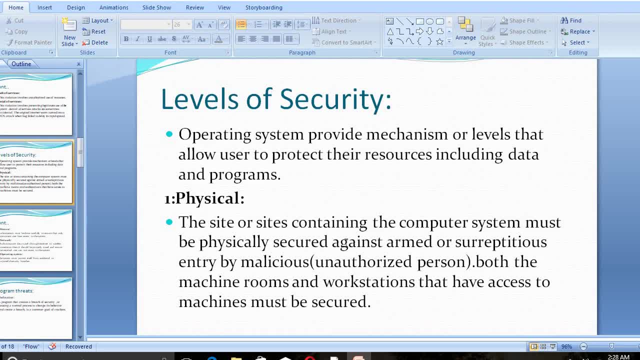 Operating system provides mechanisms or level that allows users to protect their resources, including data and programs. First level of security is physical level: The side or sides containing the computer system must be physically secured. Then level of security is physical level: The side or sides containing the computer system must be physically secured. 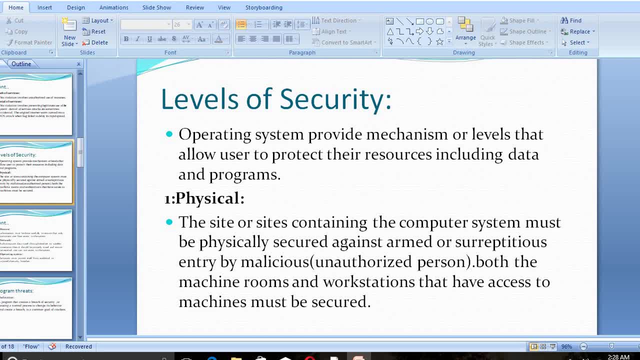 Let us consider a real-life example of a bank. like there are security guards in a bank, They are preventing the bank from entering the external user or unauthorized user. Similarly, it is very important to physically secure the operating system. Then we have email. 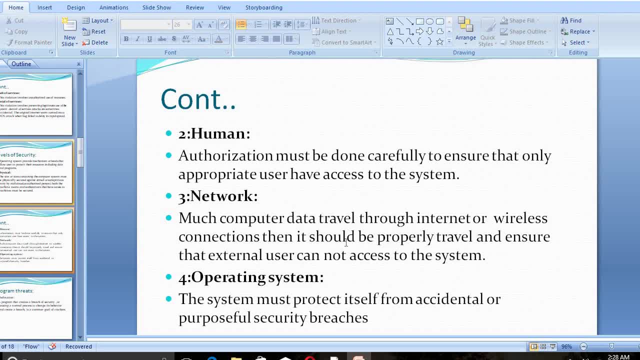 Authorization must be done carefully to ensure that only appropriate users have access to the system Means. if we take the example of a bank, then any external user who enters the bank and then he tries to access the mainframe of the software installed in the bank. 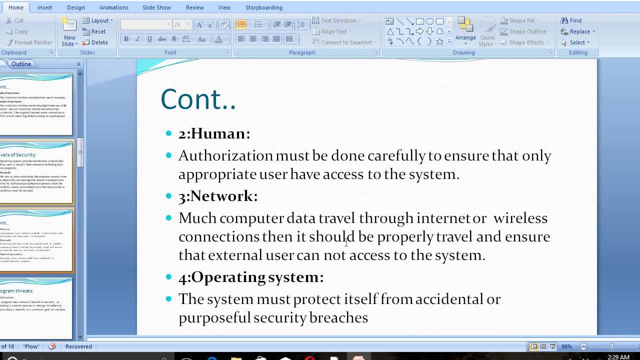 Then we have network. Much computer data travels through the internet or wireless connection. then it should be properly traveled and ensure that external user cannot access to the system. What we have here: We have a communication medium. It is very important to secure it so that no attacker can attack and damage our data. 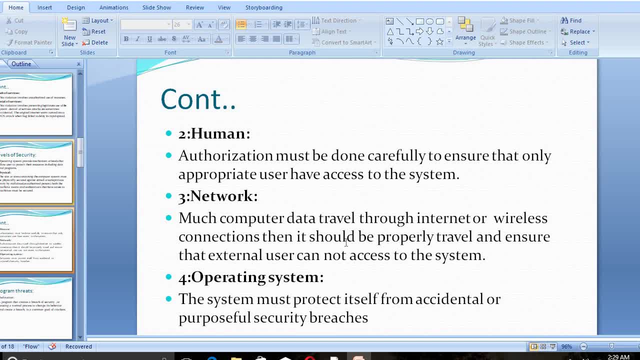 And we have data received properly from the sender to the receiver. Then we have operating system. Operating system. This system must protect itself from accidental or purposeful security breaches. Operating system automatically secures the system for itself so that no unauthorized user can access it. 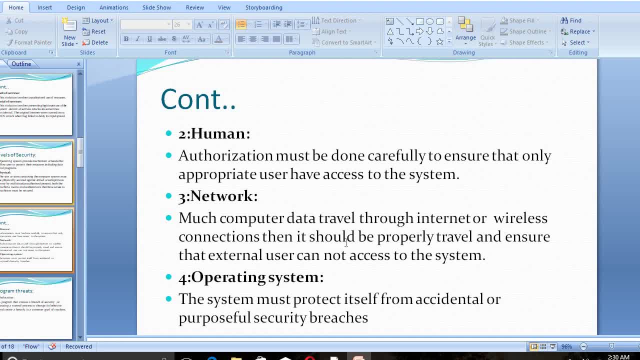 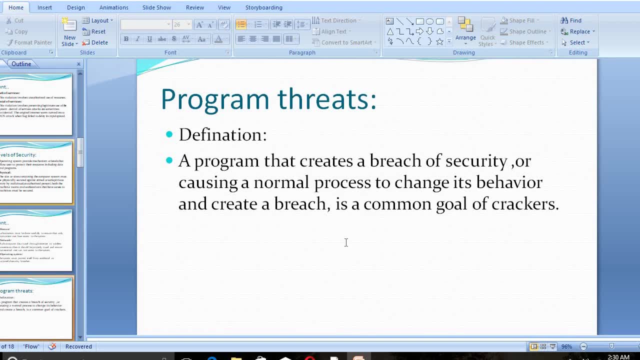 Then we have program threats. Program threats that creates a breach of security or causing a normal process to change your system, To change its behavior and create a breach Is a common goal of crackers. The program or processes that we have inside the operating system. 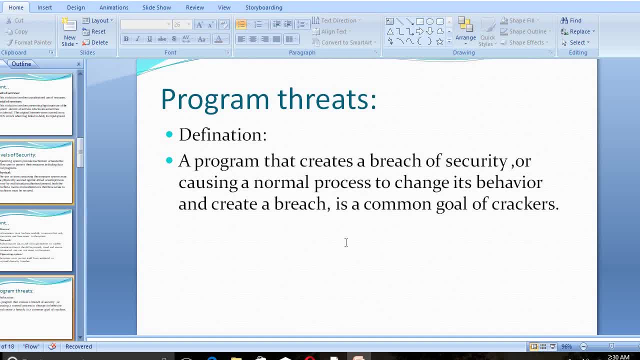 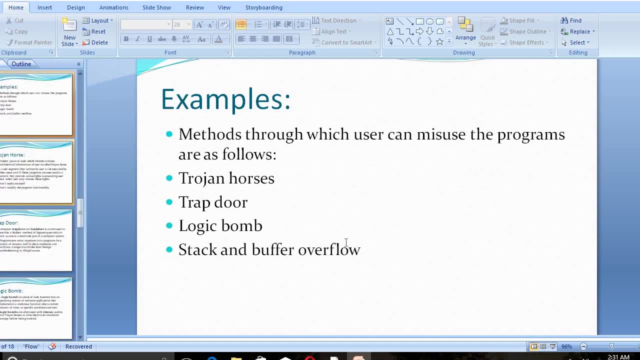 When their normal behavior changes, then we call them program threats Means their normal execution gets disturbed Through any attacker or cracker Which tries to access or damage it, So we call them program threats. Program threats- methods through which user can misuse the programs- are as follows: 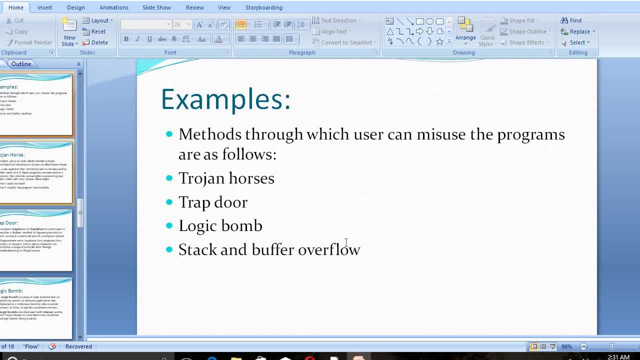 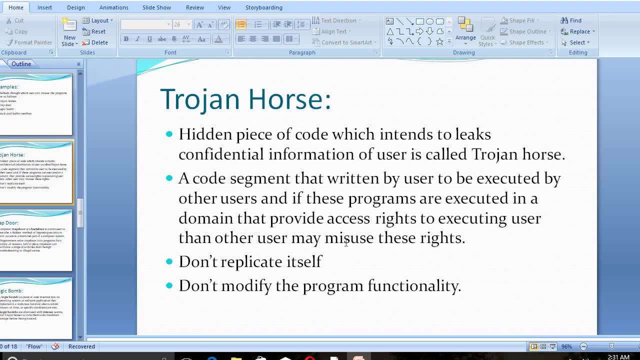 We have examples of program threats: Trojan horses, trapdoor logic, bomb stack and buffer overflow. First, Trojan horses. Trojan horses are the hidden piece of code Which intends to leak confidential information of user Is called Trojan horses. This is the code segment. 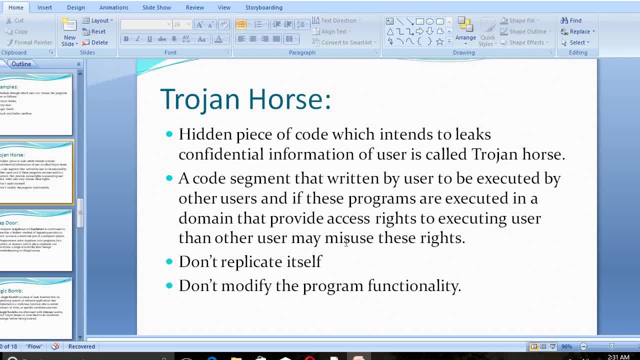 Which is created by one user And the other user uses it And all the rights are given to the user who is executing it And he tries to misuse these rights. Trojan horses, Don't replicate itself. Don't modify the program functionality. 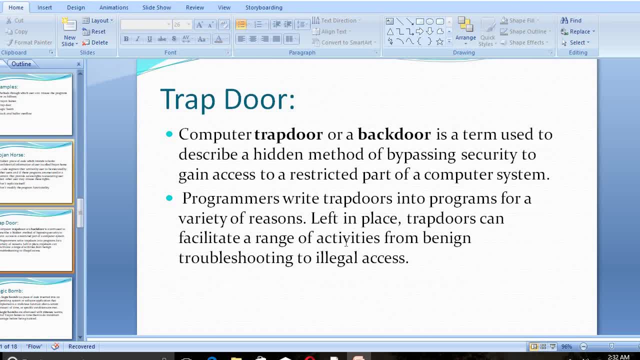 Then trapdoors. Trapdoors, also called backdoors, Means hidden methods Which tries to break the security And tries to access the system. Programmers write the code of trapdoors. There are many reasons for this: To get the confidential information of the user. 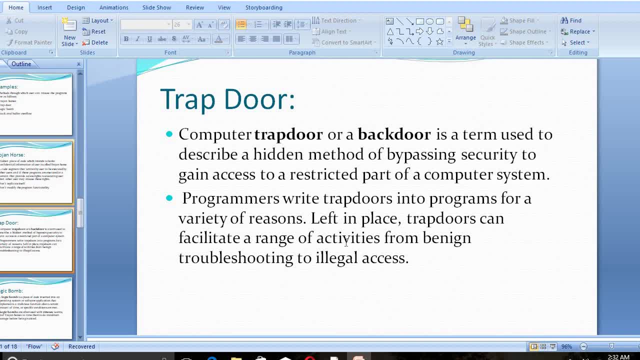 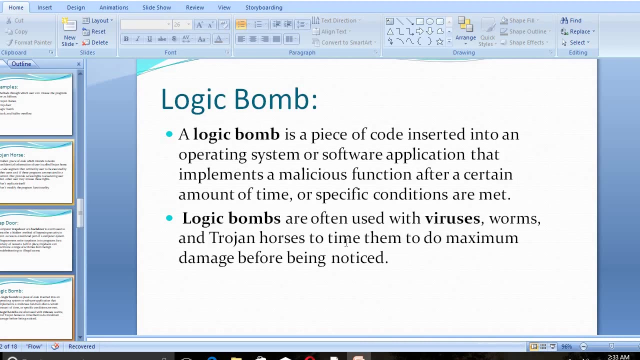 Or to access bank account numbers or credit card numbers. Trapdoors, codes are written And by breaking the security So that the system can be accessed And from there Access can be done, Illegal access is done. Then we have logic bomb. 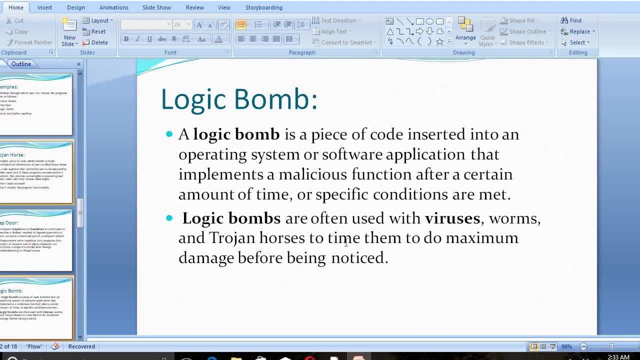 A logic bomb is a piece of code inserted into operating system Or software application That implements a malicious function After a certain amount of time Or specific conditions are made. We have this in two ways. One is that specific timer is used. 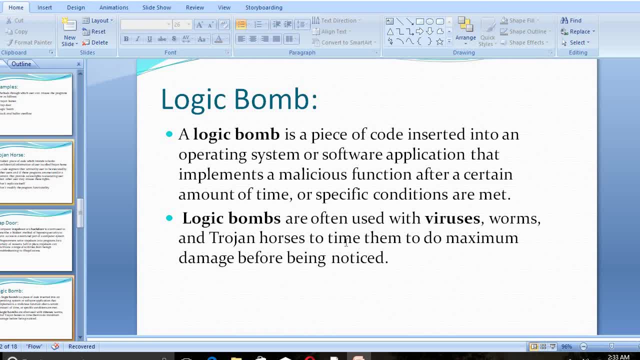 It occurs at a specific time Or specific conditions are applied. When specific conditions are met, Then these viruses are activated. And these are also activated through email Or attached to a software Or attached to a file, As soon as that file is opened. 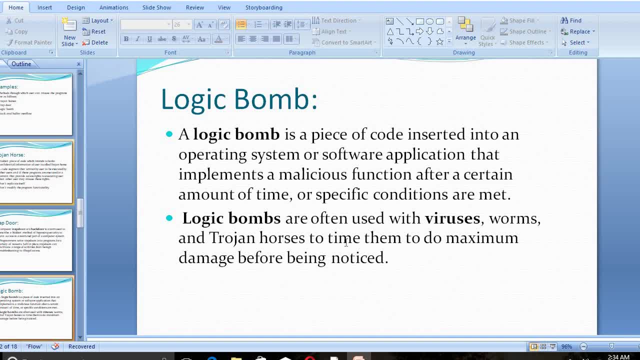 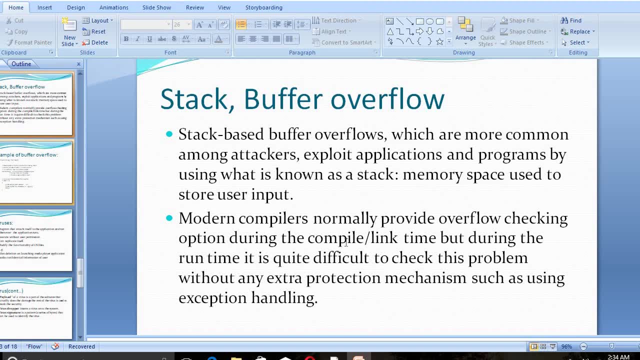 Then these viruses are entered in our system And activated. Then we have stack, buffer overflow, Stack or buffer overflow, Which are more common among attackers, Exploits applications and programs by using What is known as a stack- Memory space used to store. 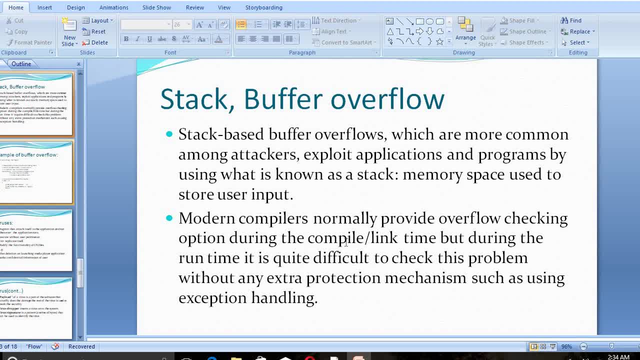 User input. Let us consider an example. For example, X program created by a user And installed on a Y machine, Then X consumes all the resources of Y, Then buffer is full. And when a process enters in the operating system And he tries to use these resources, 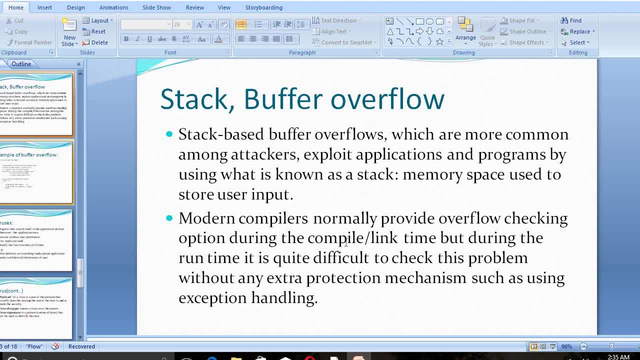 Then he can't use Because buffer is full And overflow occurs. Modern compilers normally provide overflow checking options During the compile or link time, But during the run time It is quite difficult to check this problem Without any extra protection mechanism. 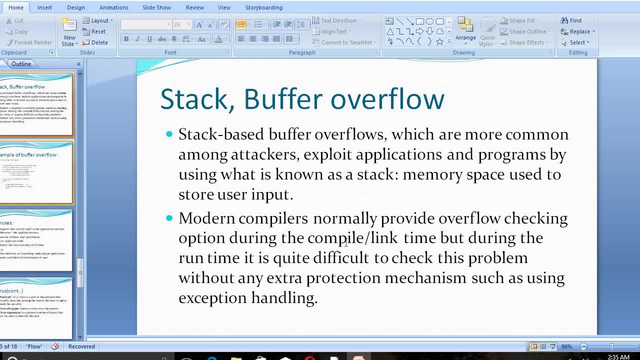 Such as using exception handling. Different compilers provide us with options So that we can check Whether there is any overflow occurring, For this exception handling concept is also used, But during the compilation It is quite difficult To check it. That the problem. 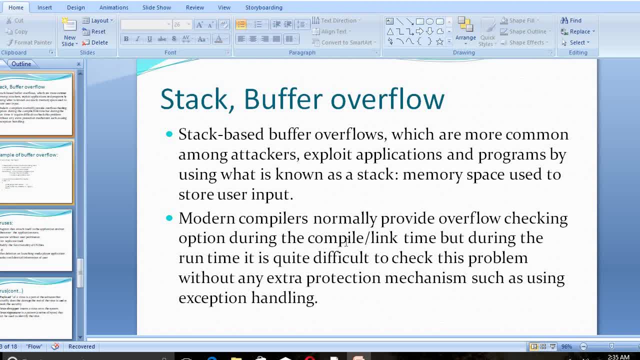 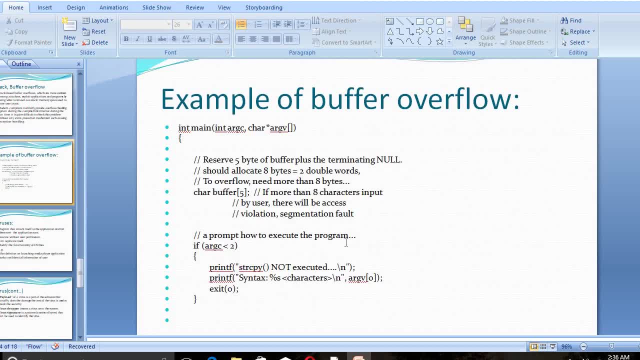 That the process is being executed, Whether there is an overflow occurring or not. Then we have an example, A code of buffer overflow is written, Which programmers write, And in this code We have A buffer is given Which reserves 5 bytes. 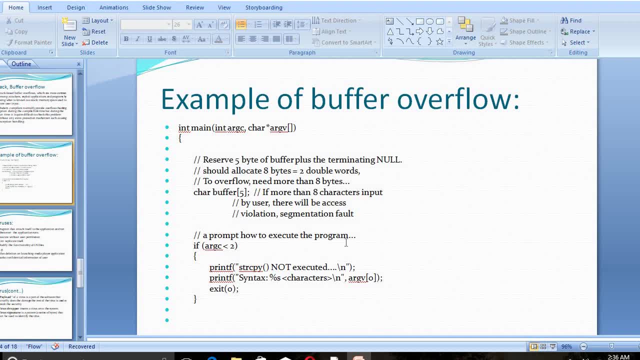 And 5 bytes Character data can be stored in it. If we input 8 characters, Then the buffer will. Then the overflow will occur. It will check the conditions When the overflow will occur When we are getting the input of 8 characters. 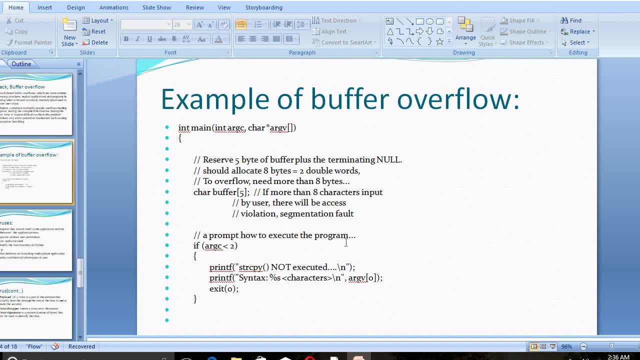 While the size of the buffer is 5. So the buffer will be full already And 8 characters. It will not store 8 characters in it. So the overflow will occur here If here, As we have given a condition, That till when the program will be executed, 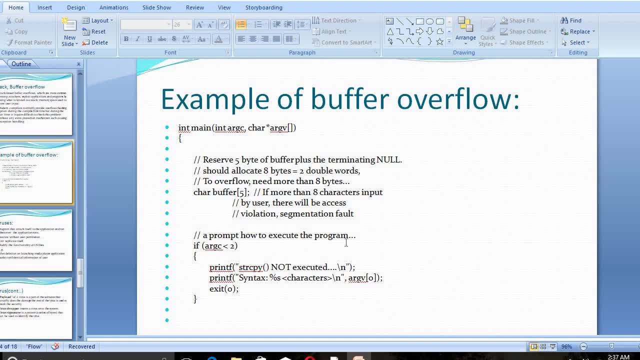 Till the condition is true. So what will happen when the condition is true? That it will call a function. That means it will not execute it And It will check the scientists, That, the characters that are coming to us, How many are coming to us? 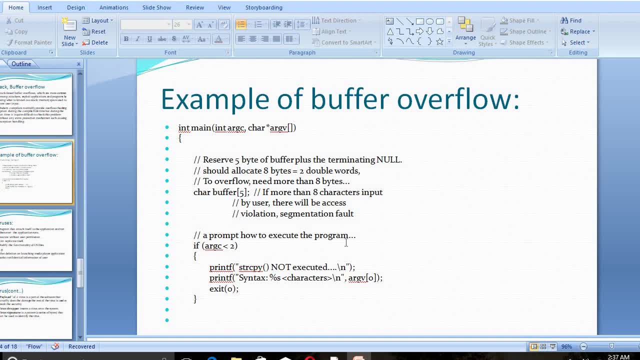 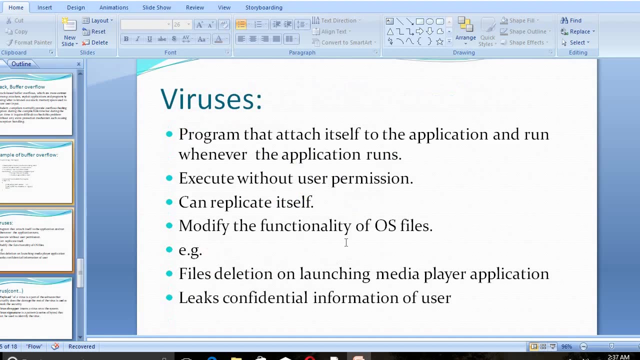 That means we have. They are stored in the buffer. So this condition is checking That the buffer Is it full or not, And then This program will be terminated. Then we have viruses. Viruses are the programs That attach itself. 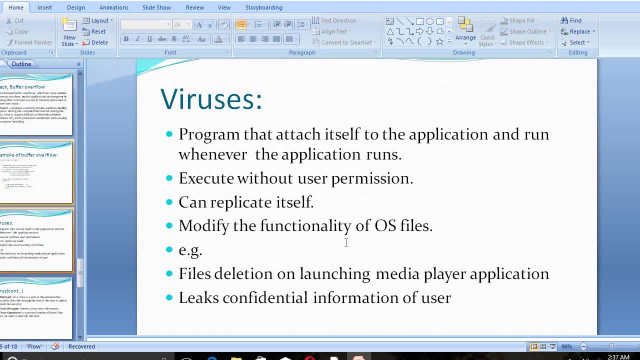 To the application And run whenever the application runs, It automatically with the program. It gets attached to any application And whenever we run the application Then it starts executing Without user permission. Can replicate itself, Modify the functionality of operating system files. 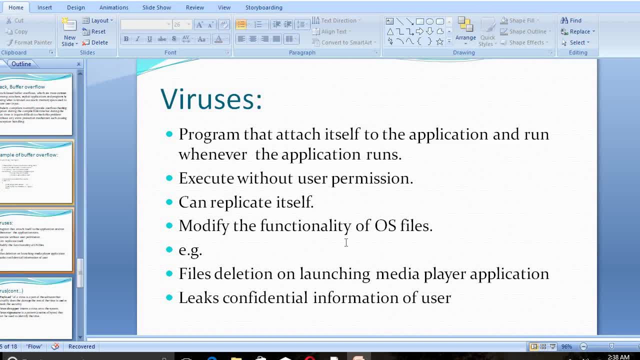 For example, Files relation On launching media player application, Confidential information, Whatever is of the user, That is also leaked, Like here. This example has been given Of media player application. If with media player application, Viruses are attached. 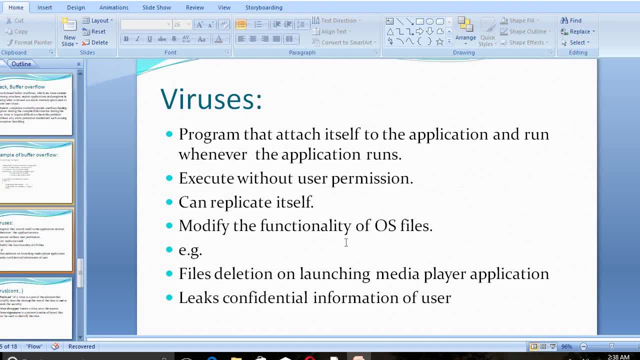 When we install this application And run it, Then automatically The virus Starts running, It gets executed, It will get activated And some media player files It will delete them. So it Damages applications, Our system Or applications. 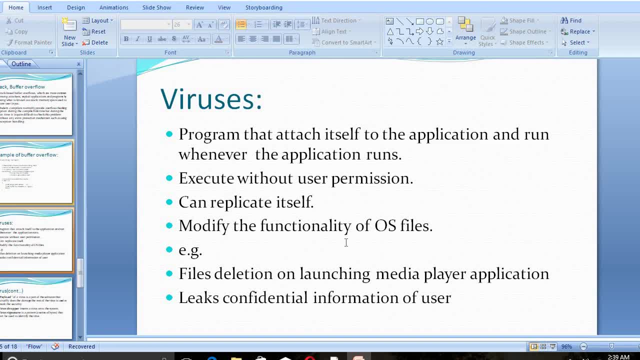 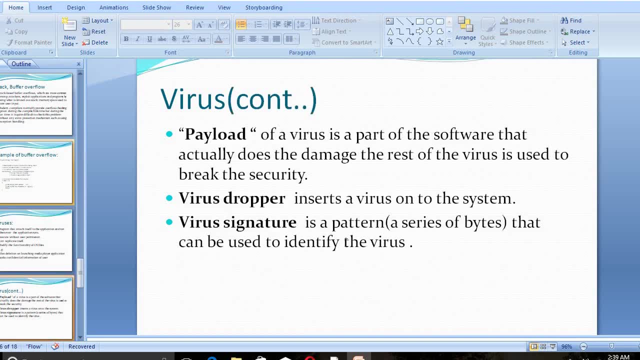 With which they are attached, They are used to damage them. Then we have Three terms in viruses: Payload, Virus dropper And virus signature. Payload of a virus Is a part of the software That actually does the damage. The rest of the virus. 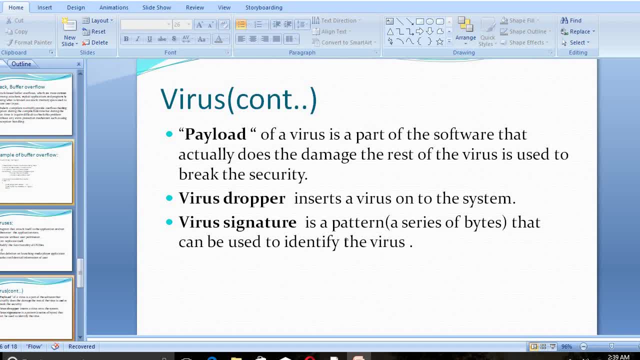 Is used to break the security. This actual Payload is that part Which our code Or our system Or software Is used to damage, And the rest of the virus Is used to break The security. Then we have Virus dropper. 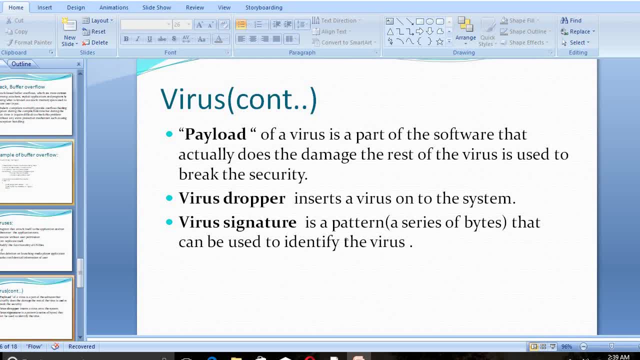 Insert a virus Onto the system. Virus dropper Is used In the system To insert The virus. Then The work Of the virus dropper Ends When it Enteres In the virus system. Virus signature. 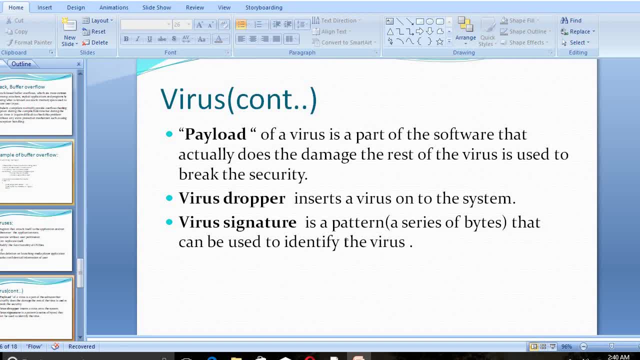 Is a pattern That can be used To identify The virus. Virus Signature Is a pattern That can be used To identify The virus. Virus Signature Is a pattern Or a series Of bytes That can be used. 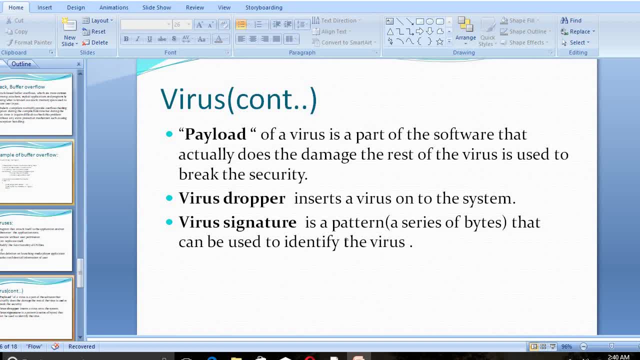 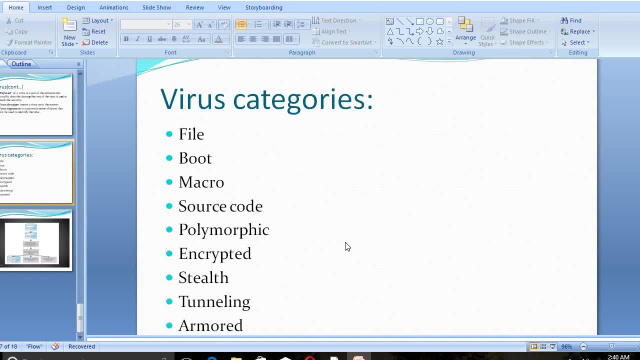 To identify The virus. Then Virus Is of Different Categories: File Boot, Macro, Source Code, Polymorphic, Encrypted, Stealth, Tuneling And armored File When The virus Is attached. 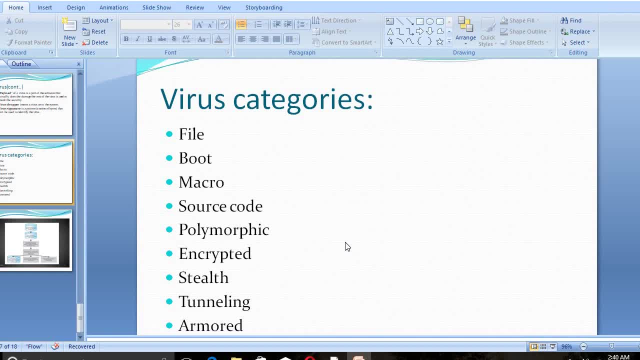 To different Files, Like Email Or Any Word File, And When We Open That File The virus Is Activated In Our System. Then Boot Is Activated. 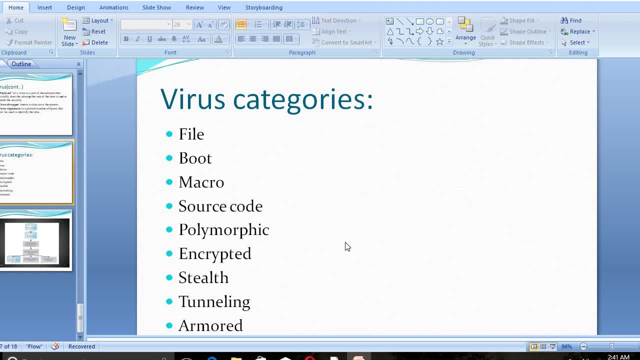 In Boot Sector. Then We Have Macro Macro, For Example, A Macro Virus Could Be Contained In A Separate Sheet File. When A Separate Sheet 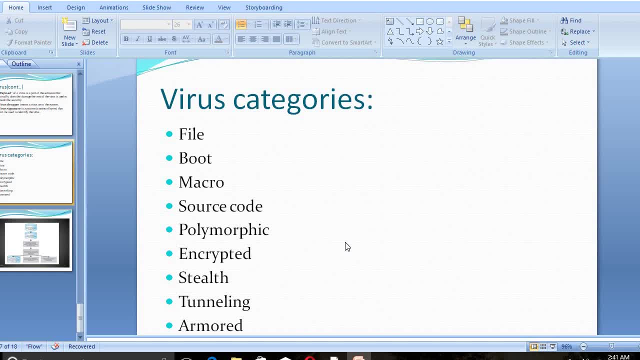 File Is Open, Then These Viruses Are Activated In A System And When We Get The Source Code Then We Modify In That And Damage. 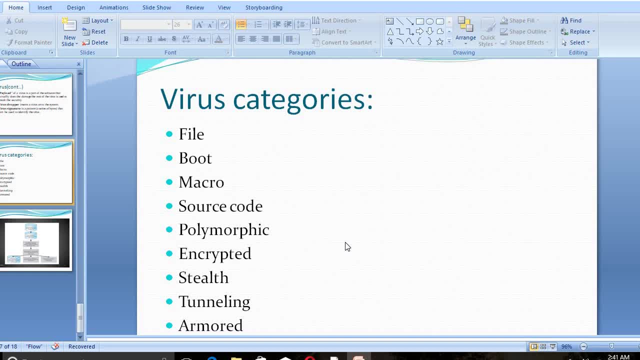 Our System Polymorphic. Polimorphic Viruses Change Each Time It Is Installed. It Avoid Detection By Anti-Virus Software. Then Encrypted: Encrypted Virus. 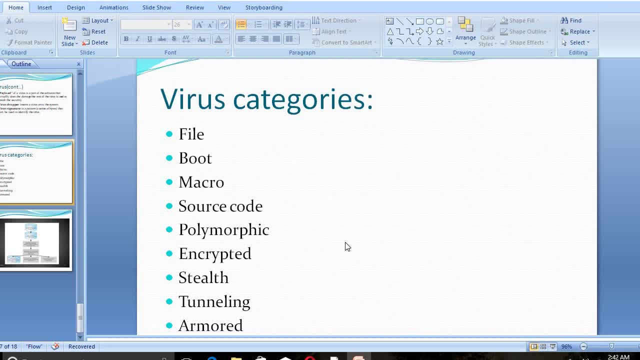 Includes The Decryption Code Along With The Encrypted Virus, Again To Avoid The Detection In This Category. First Virus Decrypts And Then Executes Stealth. 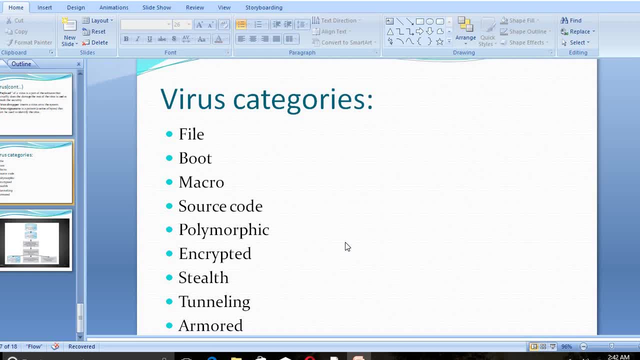 Stealth Is Attempts To Avoid Detection By Modifying Parts Of The System That Could Be Used To Detect It. For Example, It Could Modify The 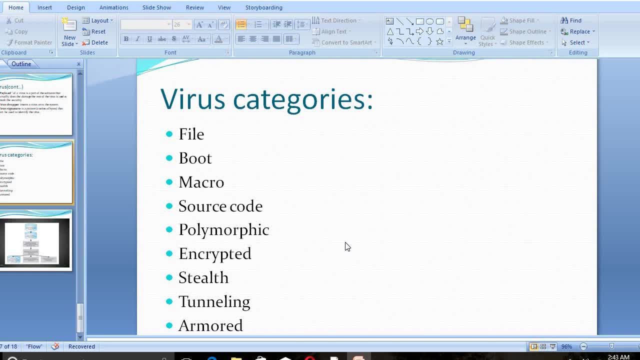 Read System Call So That If Means You Have The Code Is Modified In, The Code Is Modified And Replaced. The Original Code Is When. 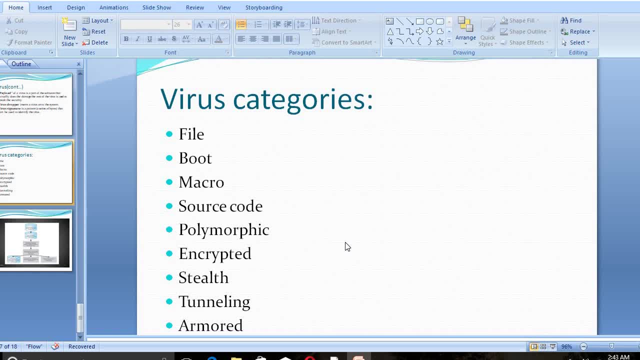 The User Open, The Code Is Modified. Code Is Infected With A Link. This Ire Attempts To Bypass Detection. An Antivirus Can A By Installing. 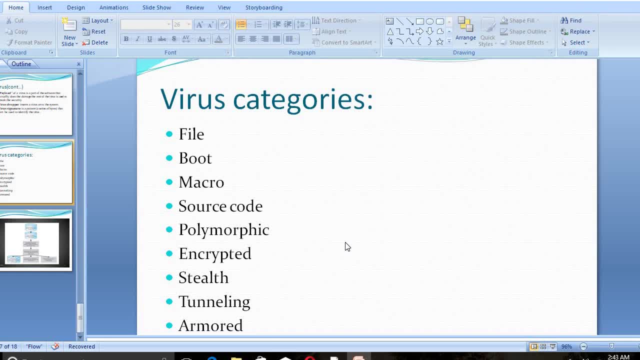 Itself In The Interrupt Handler Chain Device Drivers. Attach Втор Are Were This Is Or Act Then armored. Armored virus is coded to make it hard for antivirus researchers to unravel and understand.